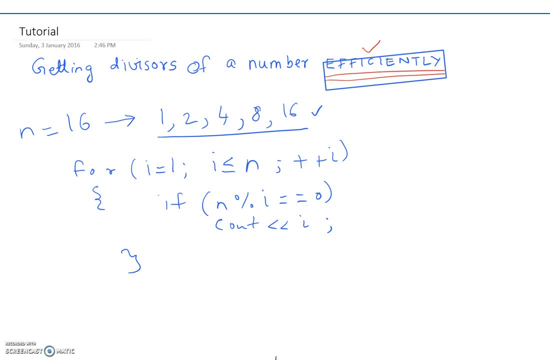 Okay, so this will be a divisor. But if I execute this code on some online platform, let's say Spodge, what I'll be getting is TLE, That is, time limit exceeded. The time taken for the execution of this program will be very high And then my program won't be getting accepted. So there is a simple solution And there is a very simple idea to this solution, which I can execute in order of root n time. 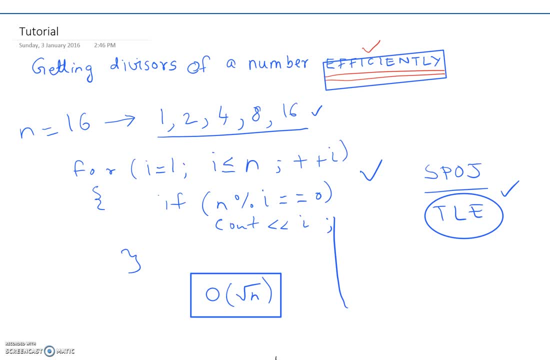 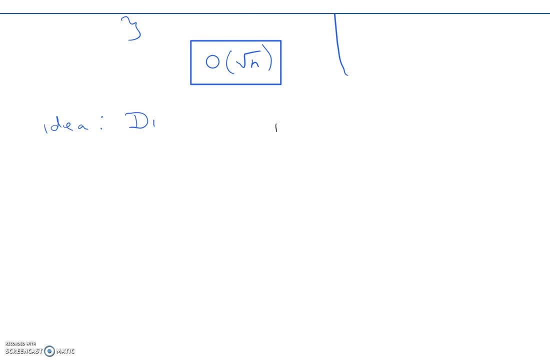 So I can use this. So now let's see the idea. Now the idea is: the idea is divisor. Divisors exist in pairs. Divisors exist in pairs. Let's say I have a number, I have a number 4. And let's say the divisor is 2. Then n by 2 will also be a divisor. 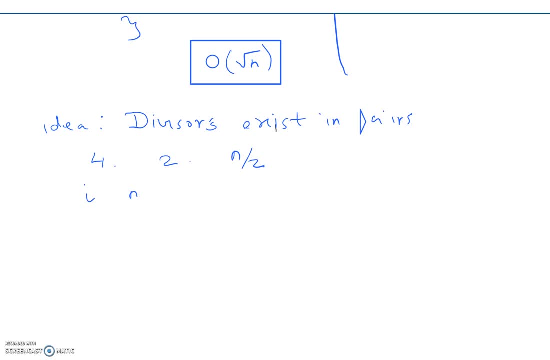 Let's say: if i is a divisor of a number n, then n by i will also be a divisor of that number n. So that is the basic concept. If i is a divisor of n, then n by i will also be a divisor. 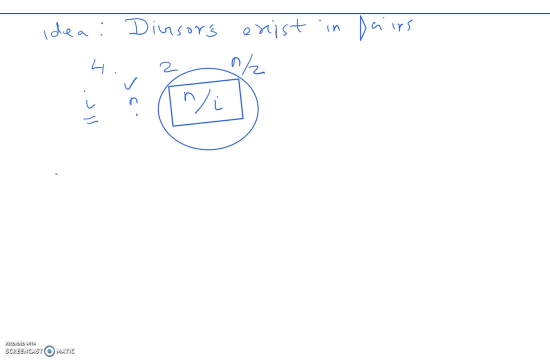 So let's see how that goes on. So I'll take the same number, 16, and I'll run this. and I'll run my loop till root n, Where n is 16. So root n will be nothing but 4. And I'll be running my loop from i equals 1 to root n. 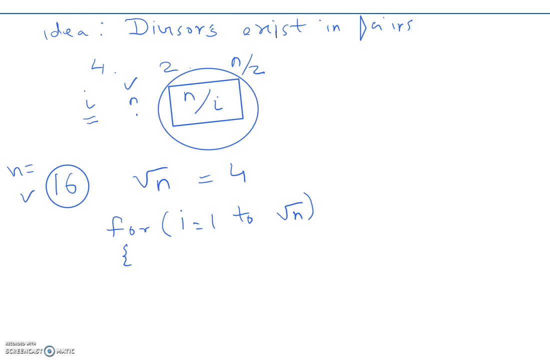 Now let's see what happens. If n by, if n mod i equals equals 0, then what I'll say: i is also a divisor and n by i is also a divisor. So what I want to say is that cout, cout i as well as n by i. 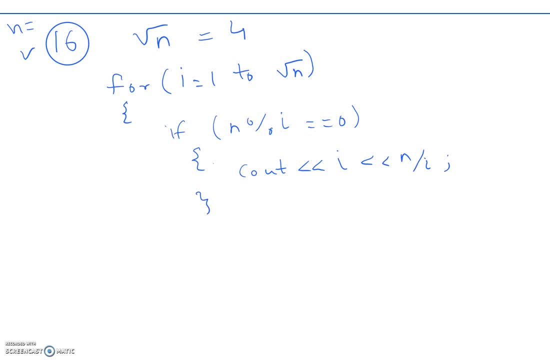 So hence I can print it Only in a time. complexity of order of root n. Let's see a basic simulation of this. 16 will be running from 1 to root n, Where n is 16.. And root n is nothing but 4.. 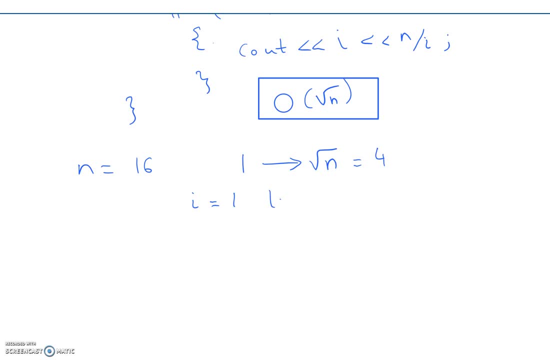 So from i equals 1 to 4.. So in the first iteration of the loop I'll be getting i equals 1.. And then i equals 1.. And then n by i. n by i is nothing but 16 by i. 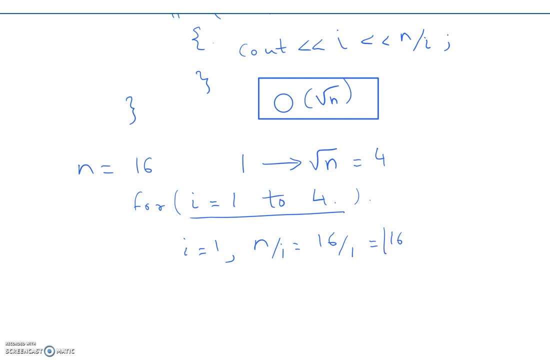 16 by i, that is 1.. So that is 16.. So 1 as well as 16 are divisors. So I get 2 divisors over here Now. in the next iteration of the loop I will become 2.. 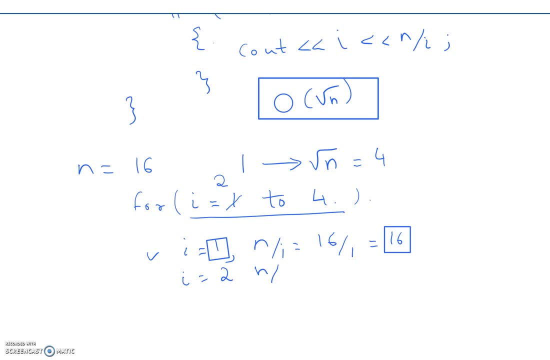 So i equals 2. And n by i equals 16 by 2.. That is 8.. So the next 2 divisors are 8 and 2. And hence so now when i equals 3.. The thing is this: 3 won't be divisible by 16.. 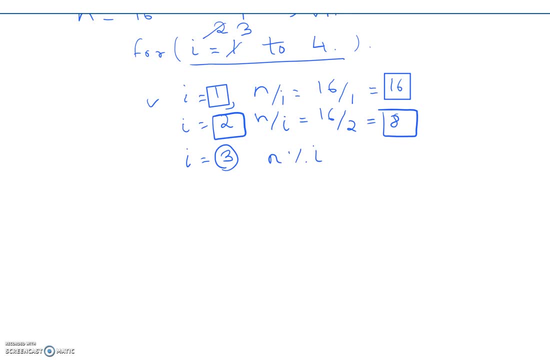 That is n mod i, That is, 16 mod 3, will not be equal to 0. So I won't proceed further in the loop Now. the next case is: i equals 4.. And n mod i- is true, That is 16 mod 4- equals 0.. 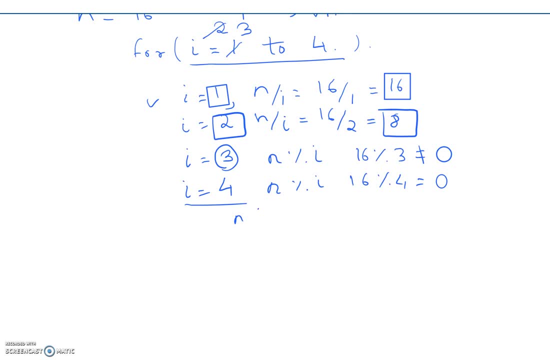 And when i equals 4, n by i equals 4.. So the 2 divisors which we get are 4 and 4.. That means they 2 are same. Now we need to put a condition and check That if i, that is 4.. 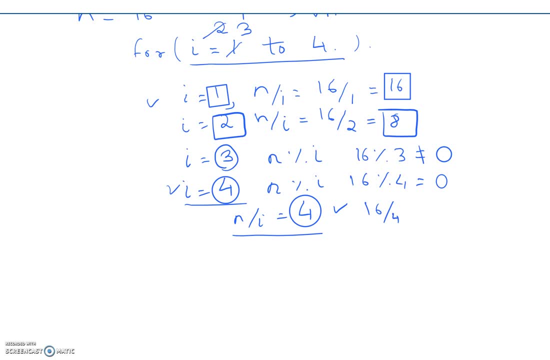 And n by i, that is 16 by 4.. If they are same, We will only print either of them, That is, either i or n by i, And hence we will only print one of them. Okay, So we can see the code over here. This is the code.